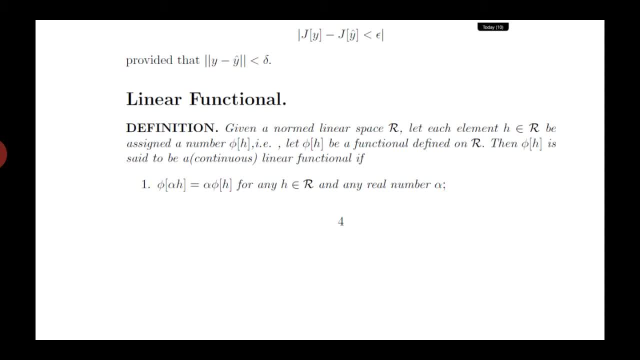 that say that, given a norm linear space, R, let each element H in R be assigned a number. phi of H, which is a functional defined on R, then phi of H, which is a functional of H, is said to be continuous linear functional if it follow the following properties. the first property says phi of alpha into H is alpha times. 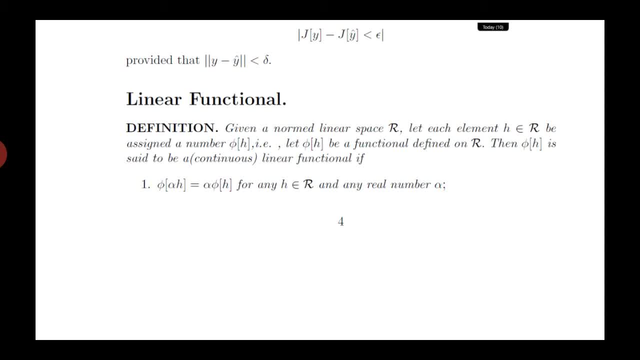 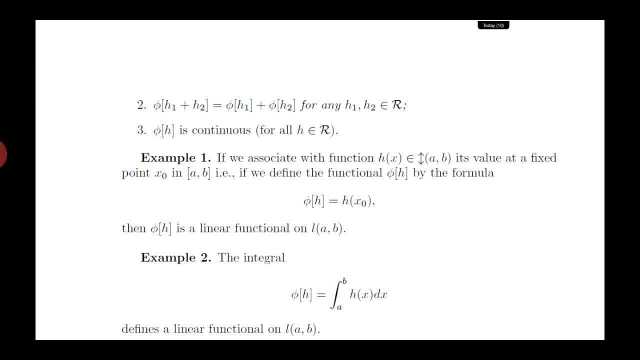 phi of H for any H in R and for any real number in alpha. the second property says that phi of H 1 plus H 2 is simply equal to phi of H 1 plus phi of H 2, where H 1 and H 2 are the element of R. and the third property says that phi of H is: 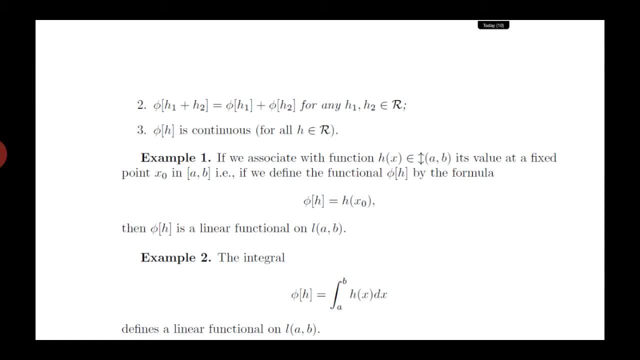 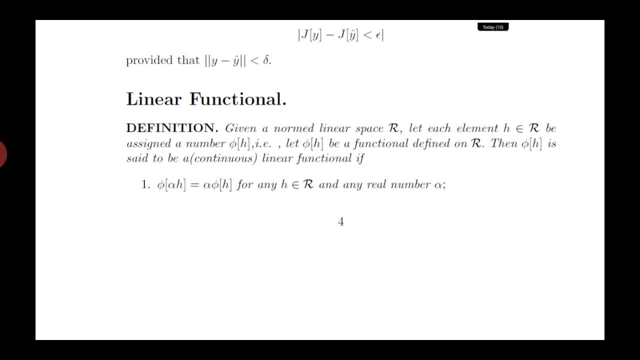 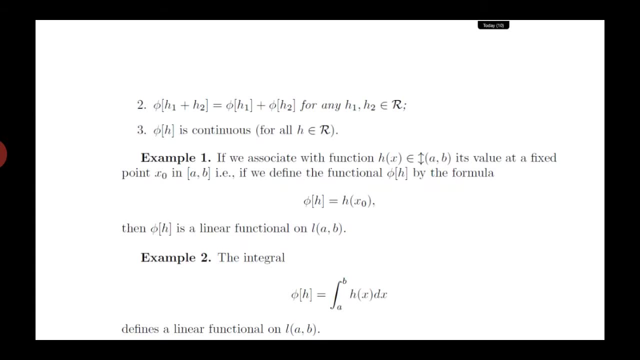 continuous for all H in R. so these are the three properties of the linear functionals and we will take a look on one by one as we go along with the examples. so let's take the first example, and this is the simplest example, and that say that if we associate each function, H of X which belongs to L of a, 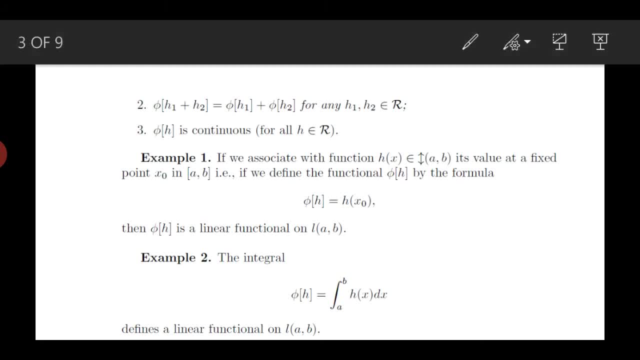 comma B, it's fixed And how we define the functional. Its value at the fixed point x0 in a b. So we take any value at point x0 that belong to interval a and b And we call this functional is equal to h of x0. It means my functional is basically the value of this function at point x0, which lie between a and b. 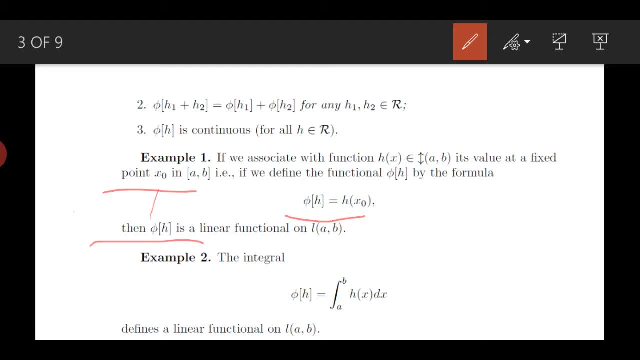 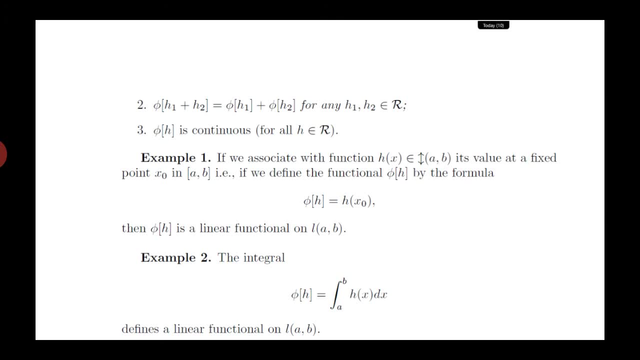 Then phi of h is a linear functional of on l of a- b. You can see whether this is following this property or not, But let's verify this by plotting some examples. You can verify it very simply that phi of alpha times h will be alpha h of x0, which can be written as alpha phi of h. And the second property is very simple, that is phi of alpha times h. 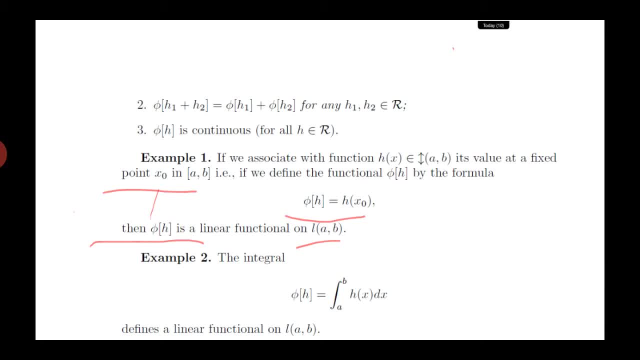 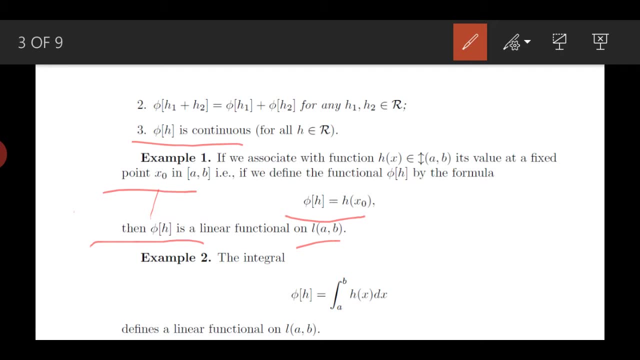 So phi of h1 plus h2 is basically h1 of x0 plus h2 of x0. And then you just write them as phi of h1 plus phi of h2.. We talked about the functional continuity in the last section and you can prove that these are the continuous. It means that if I vary my function continuously, I vary the h continuously. my functional will not vary discontinuously. It will also follow the continuity. 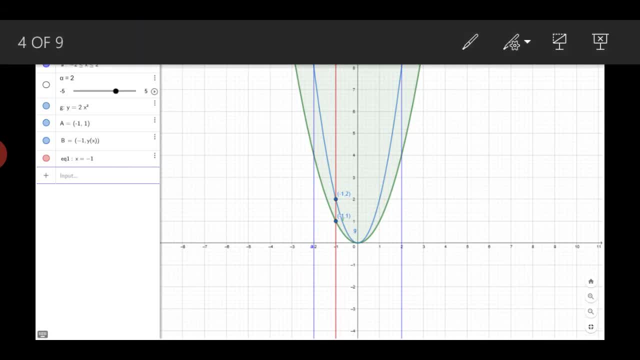 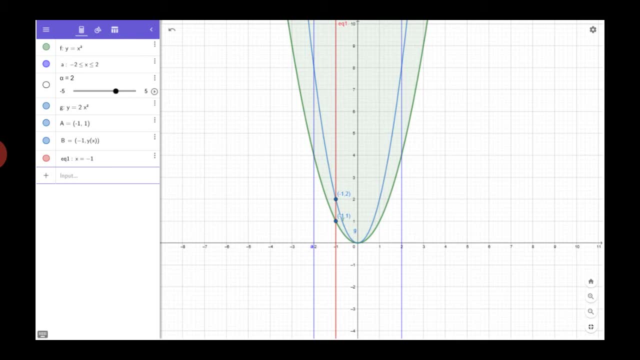 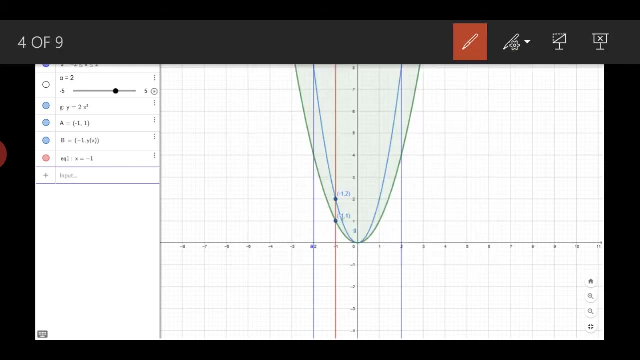 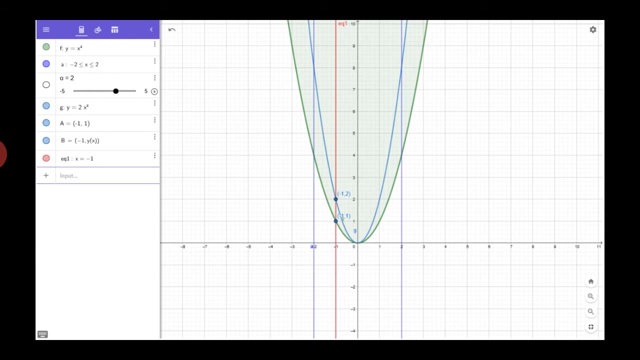 So let's take an example of that. So what I did is to plot some of the graph and what I take as an interval is from minus 2 to plus 2.. And I plot first one is my parabola, that is, y is equal to x square. And then I plot, I multiply it by the n number to follow the first property, that was phi of alpha times: h is equal to alpha. 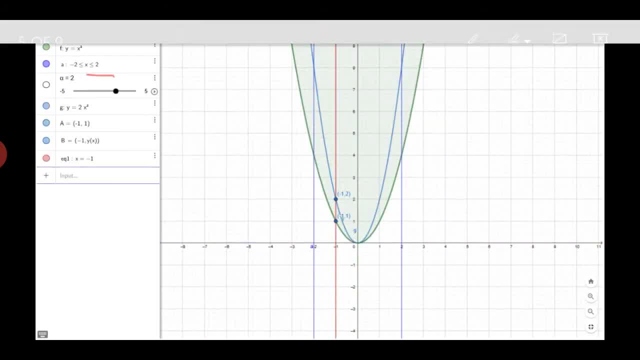 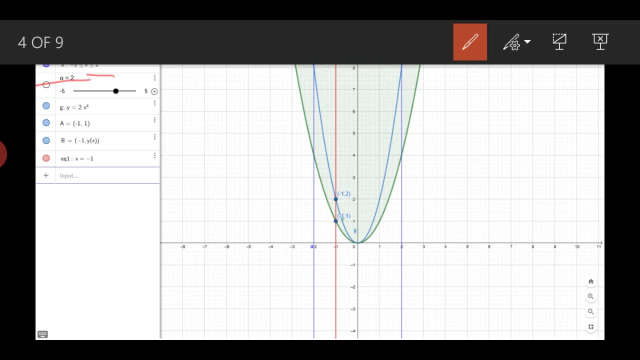 So what I did is to multiply this function x square by a number, alpha, and I write alpha as 2.. I assign alpha value to be 2.. So my function will become: y is equal to 2x square. So there are two graph: The green one will be x square and this blue one is 2x square. 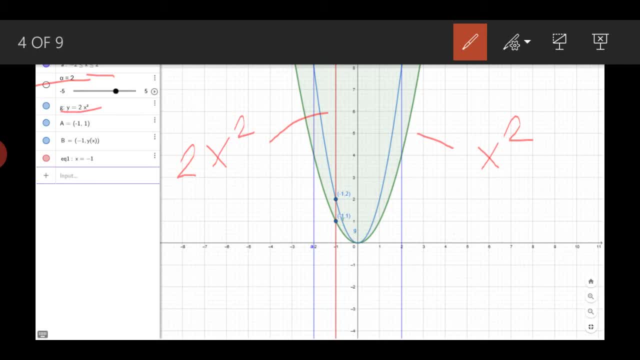 Then at any point I can write the functional. I define a functional by the value of this function at some point, and I take this point to be minus 1.. So the first one have a value at minus 1 comma 1.. It means that its value is 1.. And the second one is minus 1 comma 2.. It means that if I multiply this point by 2, then I get this one, this value. 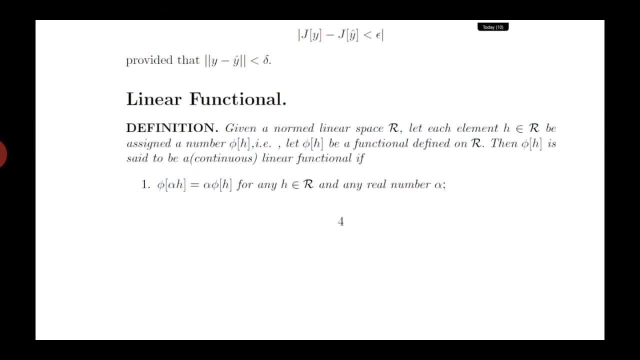 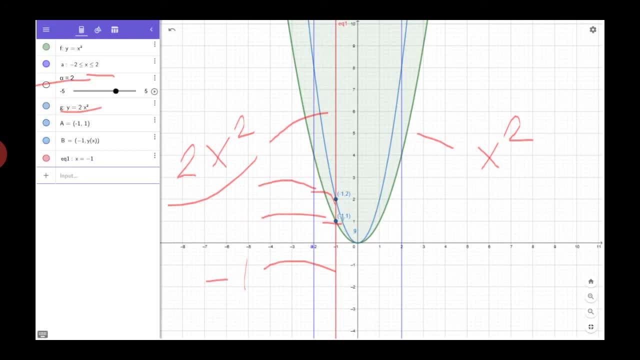 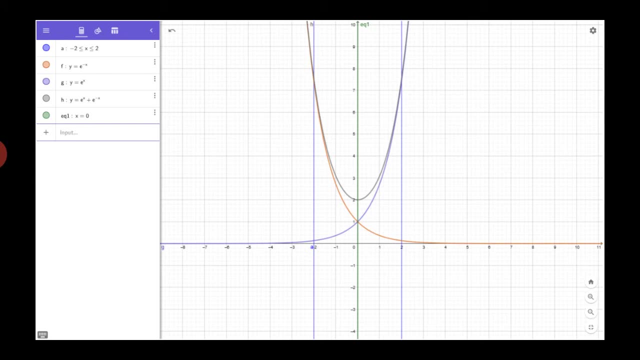 And that's the first property- said That phi of alpha comma h is simply multiply phi of h by alpha. So this can be verified by the simple example. Let's take a look on the second example. For the second one I take the same interval, that is, minus 2 to 2.. 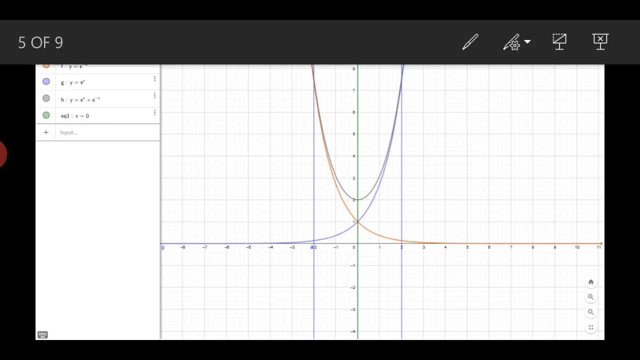 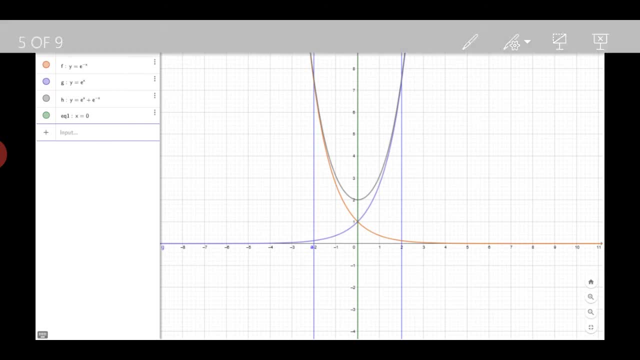 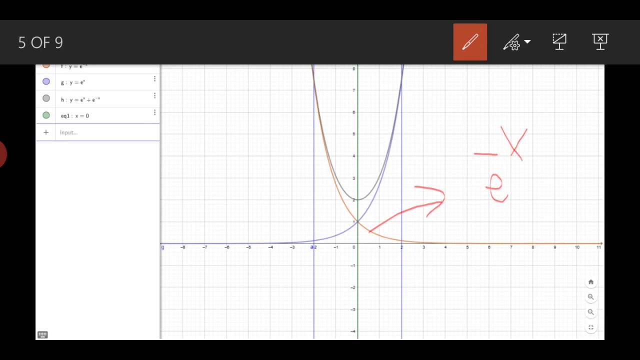 And I define two functions: y is equal to e to the power minus x, and y is equal to e to the power plus x. So this orange one, This orange one, is basically e to the power minus x, And this purple one is e to the power x. 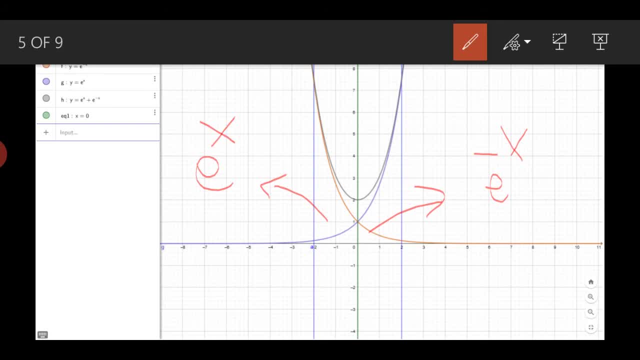 And what it says: that if I define a function like y is equal to e to the power, some of these function And this one, this graph is basically showing you the graph- of y is equal to e to the power x plus e to the power minus x. 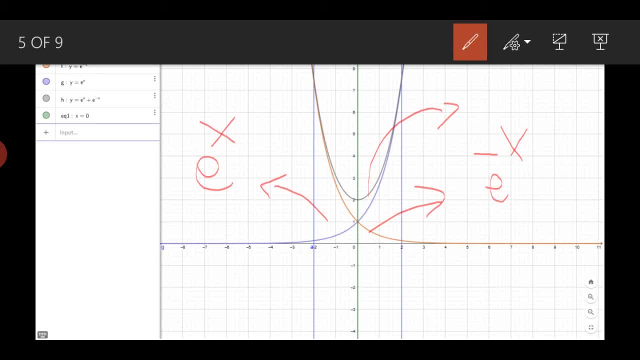 Then I can write my functional as specifying the value of the function at some point, And in this case I choose this one to be 0. So I choose x naught to be 0. The value of the first one is 1.. 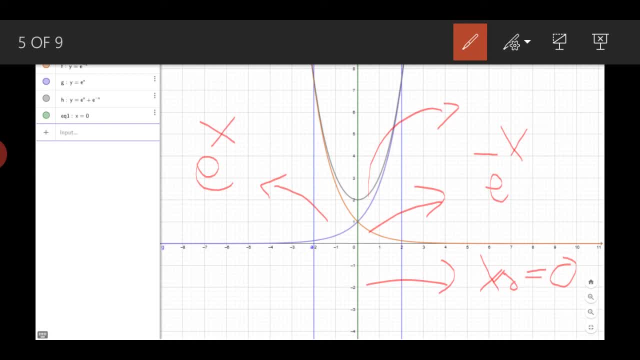 And the second one is 1.. And some there, some have a value of 2.. So you can see that if I add both of them, 1 plus 1, and that is equal to 2.. So this is the second example of the second one. 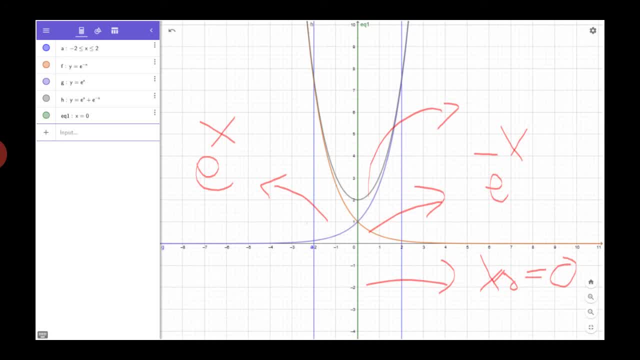 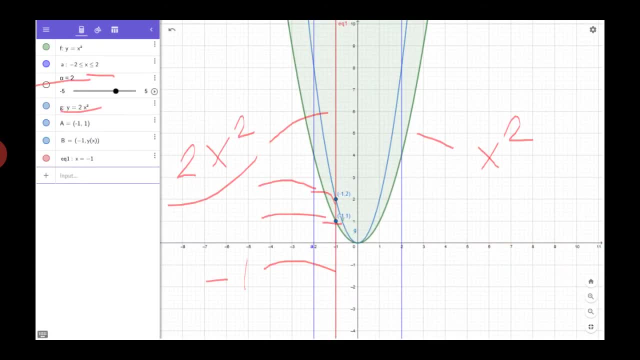 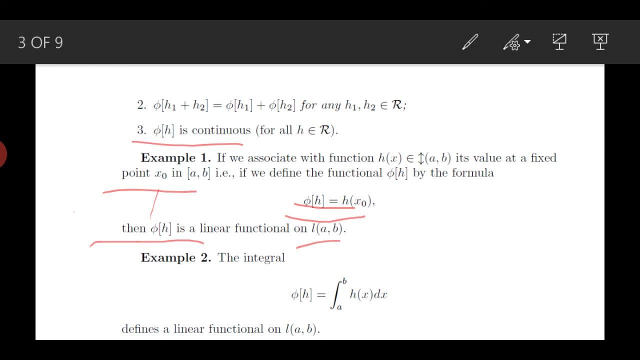 So this is also following the linearity. Let's talk about the third one. We will not discuss the third one because it is a little bit confusion. So we will go on to the second example and that is the integral. The integral is also a linear functional, or you can also say it is a linear operator, because you can write the function. 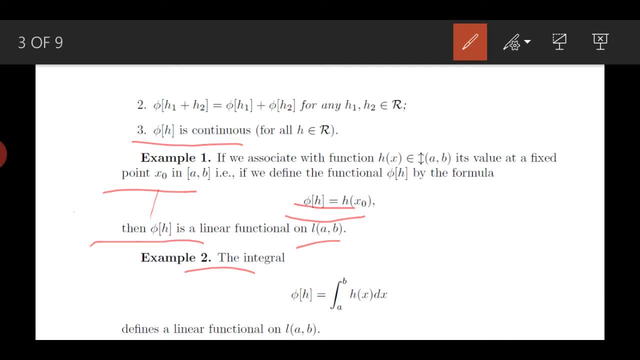 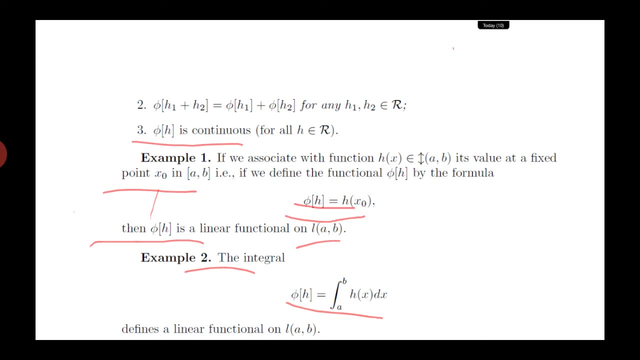 in plus, if the function is h1 plus h2, you can write it as integral h1 plus integral h2.. So this one is also a linear functional and you can show this rigorously. But we will look at the example and see some intuition. 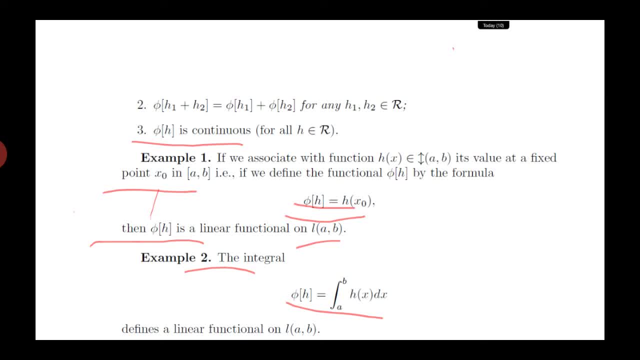 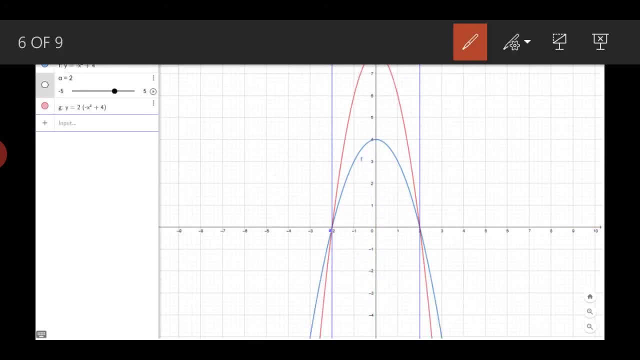 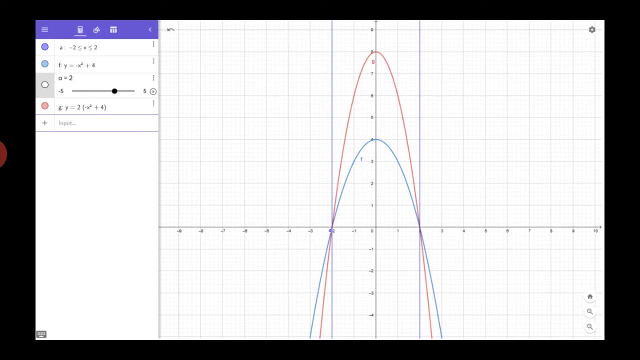 In the more general case we will prove how to prove these two, one and the more general case. So let's go into the slide And let's plot two functions. The first function is: y is equal to minus x square plus 4, and that is represented by this blue one. 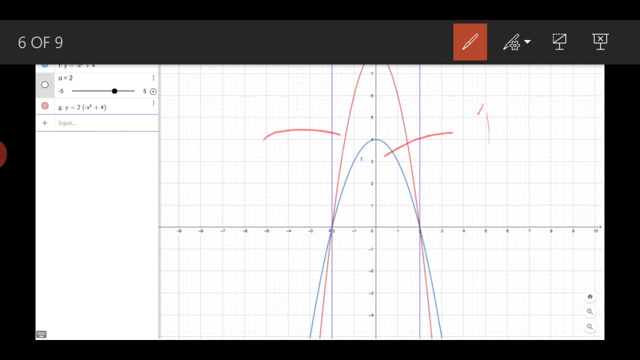 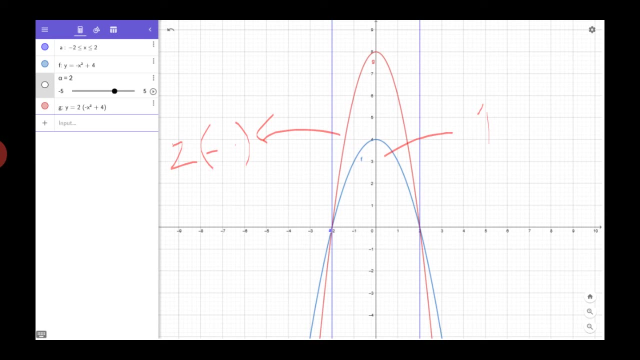 This is the first one, and the second one is basically the two times of the first one. So I multiply the first one by 2.. Then you can see that if I did this, then the area is also get double. So as an exercise, you can find out the area between first one and the second one and you will see that 2 is a. 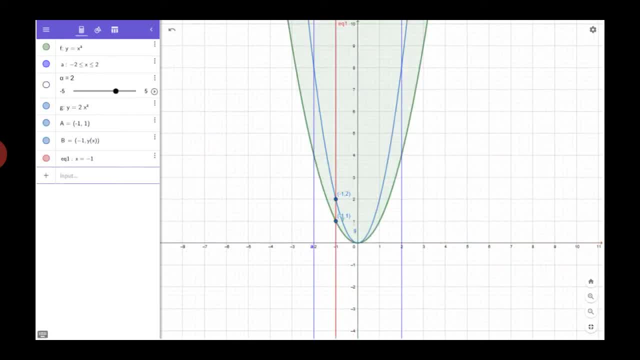 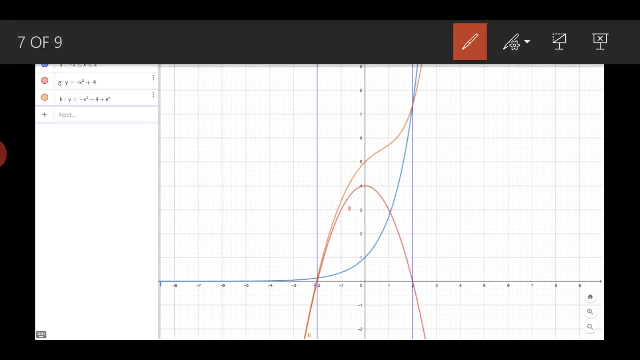 multiple. So that is the same thing as the first property. In a similar way you can verify the second property and that says that if I find out the area under this curve, which in this case is minus x square plus 4, and then I find out the area under this curve, and when I 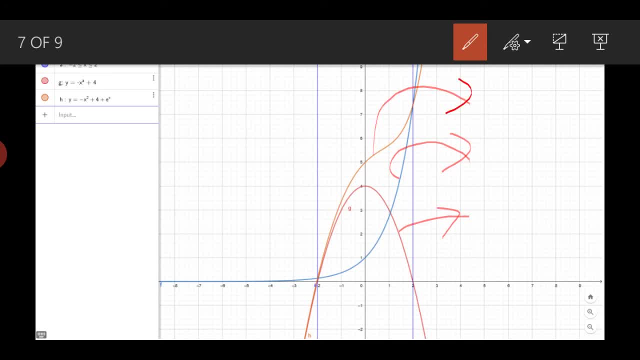 add them, that will add it to the area of this curve, which is the sum of both of them. So this is the second property, Which says that phi of h1 plus h2 is phi of h1 plus phi of h2.. 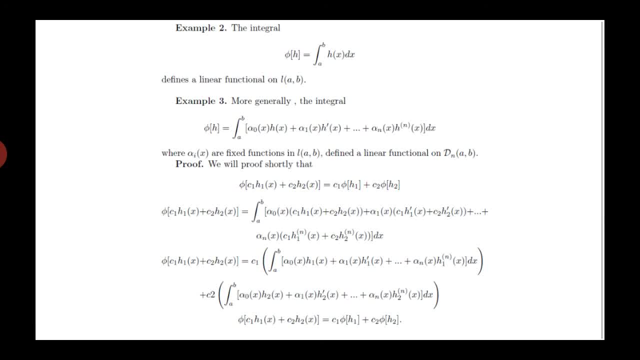 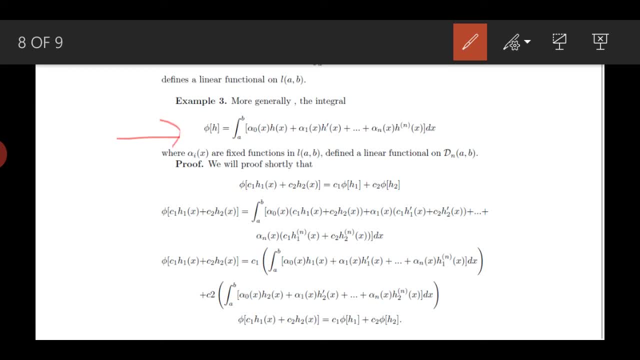 So let's go back to the more general case. and the most general case of the linear functional can be written as: phi of h is equal to integral from a to b. alpha of 0 of x, h of x plus alpha 1, dot, dot, dot and so on. 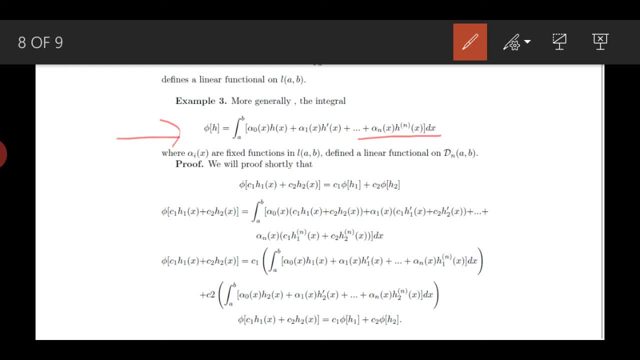 Where h, prime of x, is representing the first derivative of h And h of n is representing the nth derivative, and this function, alpha 0 of x, alpha 1 of x and so on, are basically the field function in l of ab and this functional is basically defined on dn of ab, because we have to 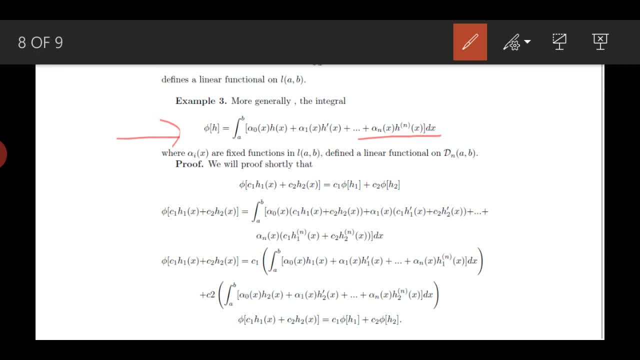 choose a functional space where the nth derivative of the function is defined, and that is my dn of a comma b. Now to prove the first and second property, we can write them in a combined form, and that is writing that phi of c1, h1 plus c2, h2 is equal to c1, phi of h1 plus c2 phi of h2.. 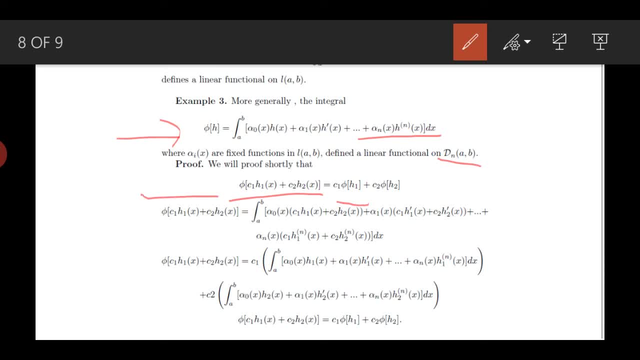 So I can write the first property and the second property in a combined form, because according to first property I can write this function as phi c1, h1 plus c2, phi 2. H1 plus Phi- C2, H2, and by the first property I can take out the constant. 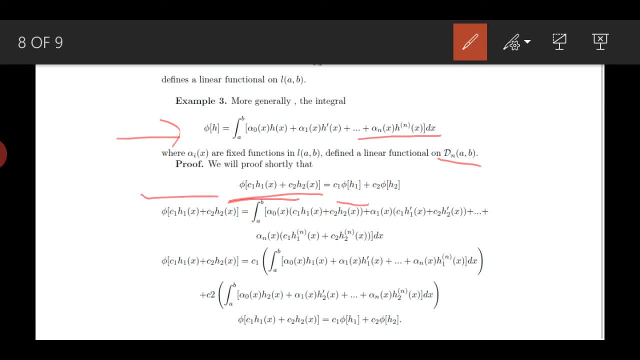 terms C1 and C2 outside the functional, and I get C1, Phi of H1, plus C2, Phi of H2. so how can I prove this is by taking the left-hand side, and when you take the left-hand side, what you get is to write this by definition of this functional. 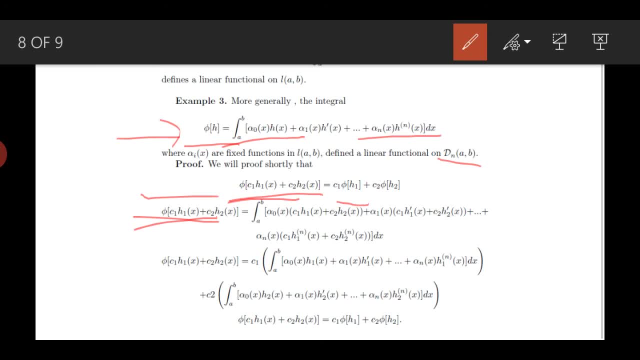 as in this form. so in place of H, of X, I will write C1, H1 plus C2, H2. and what I did in this line. you can pause and ponder. what is this written in a second line? what I did is to write the H1 term on a one bracket and H2 term on a. 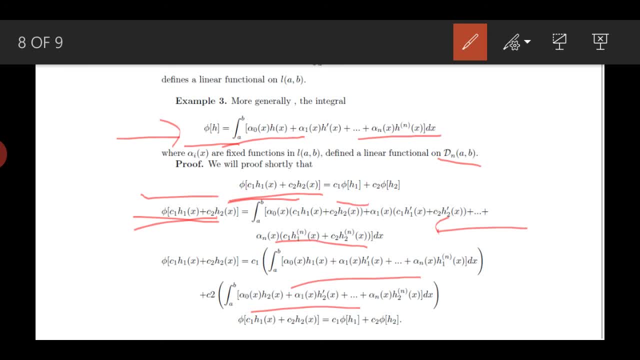 second bracket, so all the H1 term will be in one side and all the H2 of X term will be on a one side, and as C1 and C2, c2 are common, i can take them outside the integral, and what i get in this bracket is just: 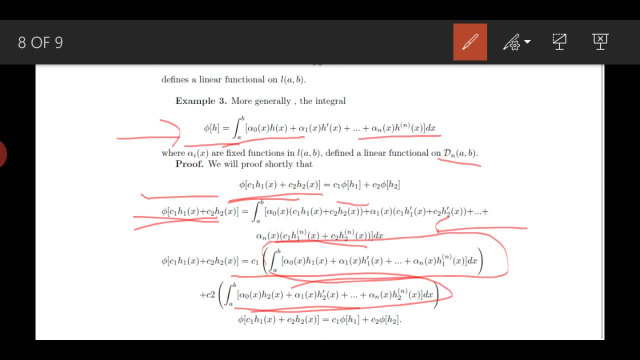 phi of h1, and what is in this bracket is phi of h2. so what this become is c1 phi of h1 plus c2 phi of h2. so this is how you can show this more general form of the linear functional and in a 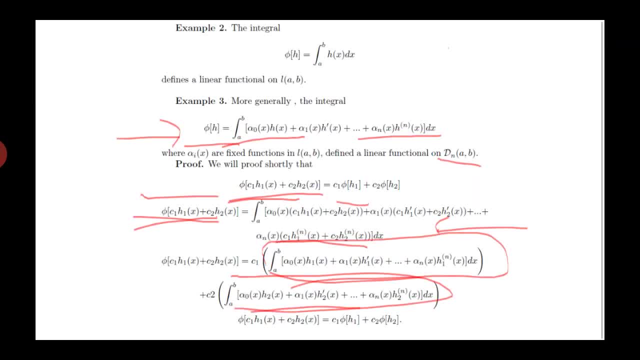 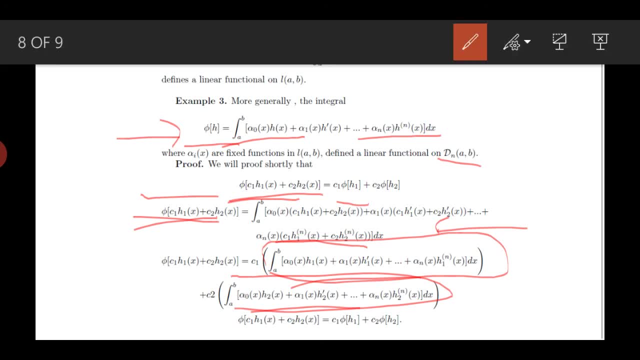 similar way you can prove the other one. the first one was a constant and the second one was just a first term in a second, in the in second example. all you need to do is to put these term equals to zero. it mean alpha 1 of x, alpha 2 of x and alpha n of x are identically equals to zero. 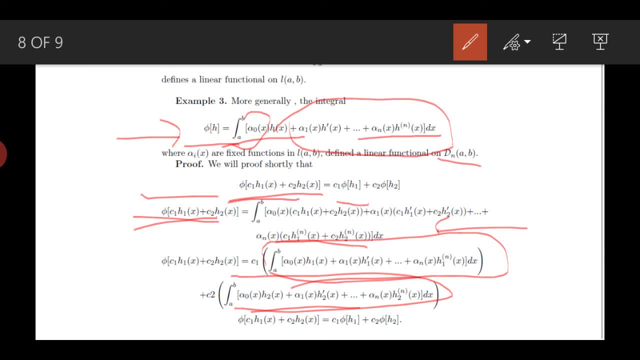 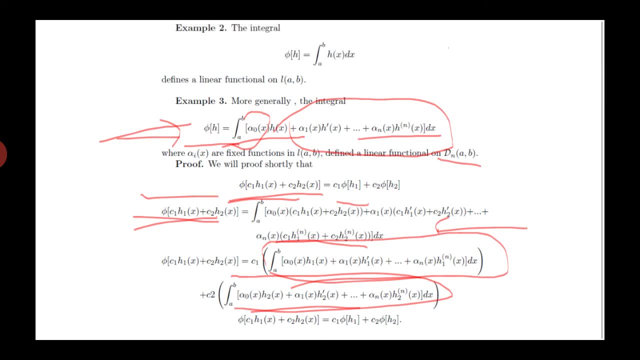 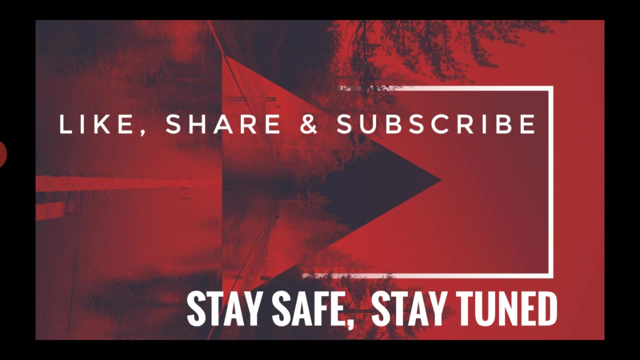 and alpha naught of x is basically one. you can see that this is more general case and we will prove other with the help of this. so this is what linear functional mean. we will see in a next video what mean by the variation of functional. it mean the derivative of the functional. so stay safe, stay tuned.